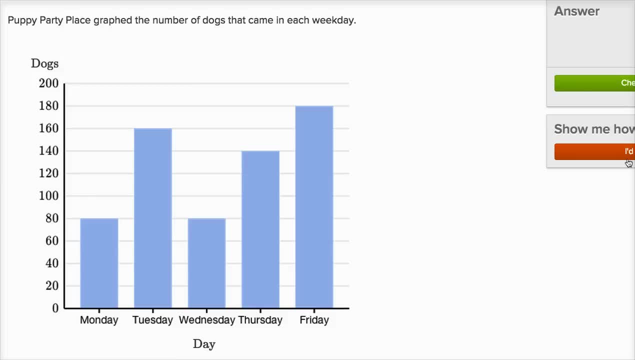 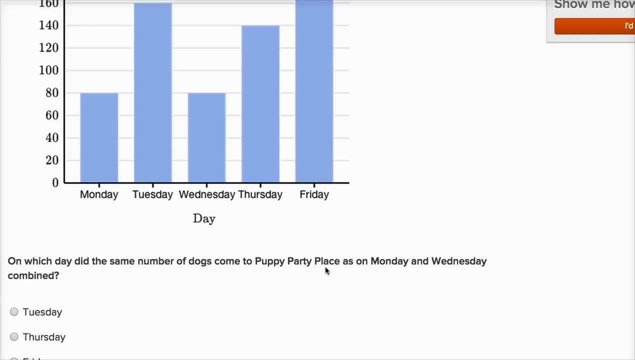 180 dogs came into the puppy party place on Friday, All right. so what are they asking us? On which day did the same number of dogs come to puppy party place as on Monday and Wednesday combined? All right, so let's see. 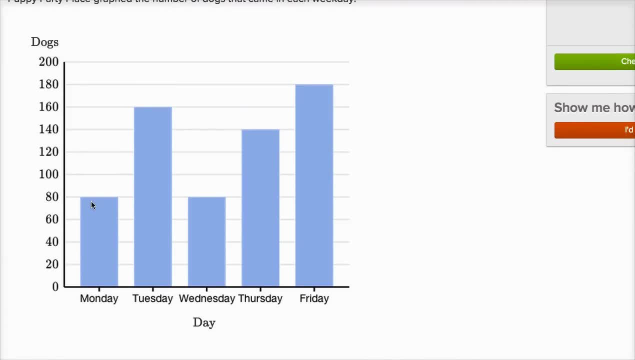 Monday and Wednesday combined. So on Monday we had 80 puppies come there, or 80 dogs, And on Wednesday we had 80 dogs And they're saying which day had the same as Monday and Wednesday combined. So Monday and Wednesday combined would be 80 plus 80,. 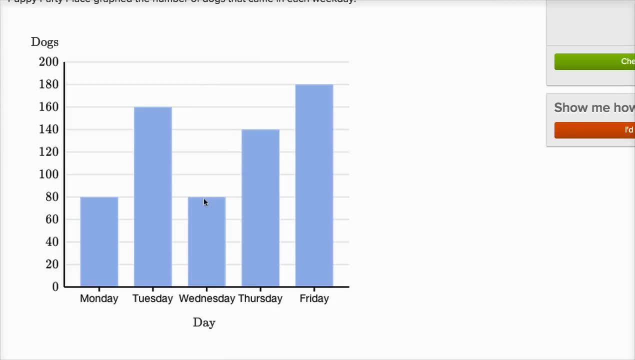 which would be 160.. So on which of these days is it 160 dogs? Did 160 dogs come? Well, we see it right over here: 160 dogs. that was on Tuesday, And only on Tuesday. So Tuesday, Let's do a few more of these. 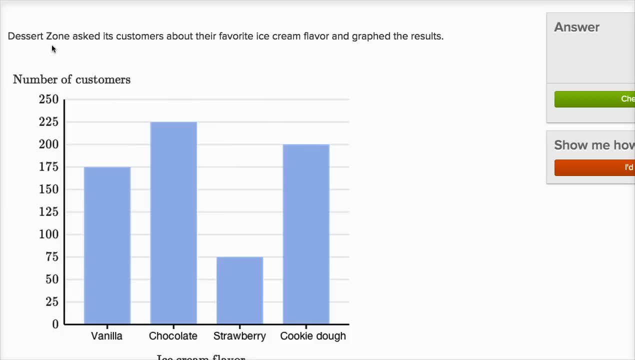 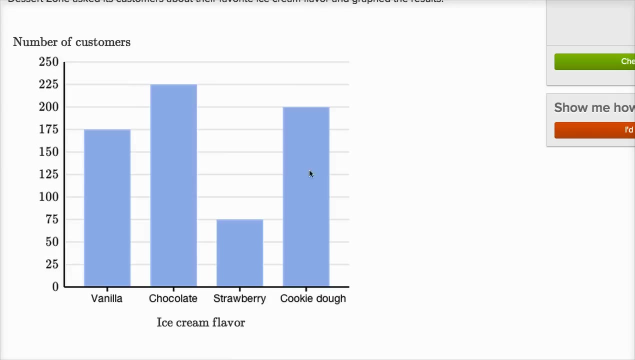 Dessert Zone asked its customers about their favorite ice cream flavor and graphed the results. So 175 customers said vanilla, 225 said chocolate, What was? 225 said strawberry And 200 said cookie dough. All right, how many more customers? 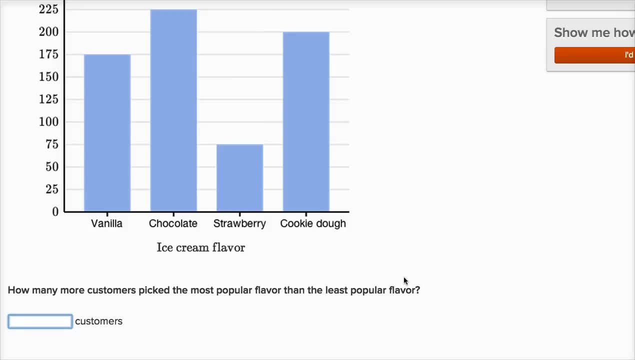 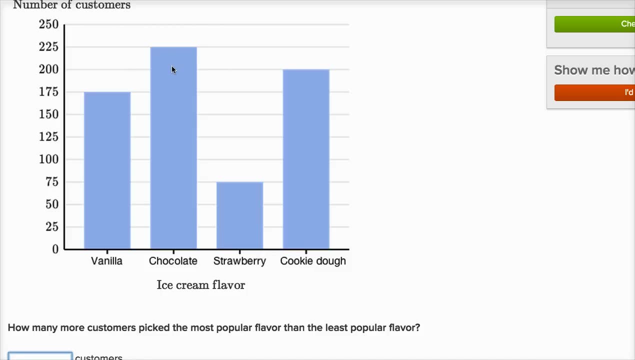 picked the most popular flavor than the least popular flavor. All right, so the most popular flavor was chocolate. That was 225.. And the least popular flavor- it's late to the least popular flavor- it's a tongue twister- was 75.. 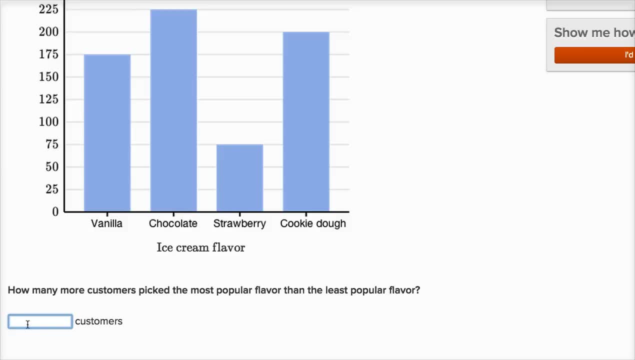 So how many more picked the most popular than the least popular? Well, the most popular is 225.. The least popular was 75. So it's 225.. So it's 225 minus 75.. Let's see, 225 minus 25 would be 200. 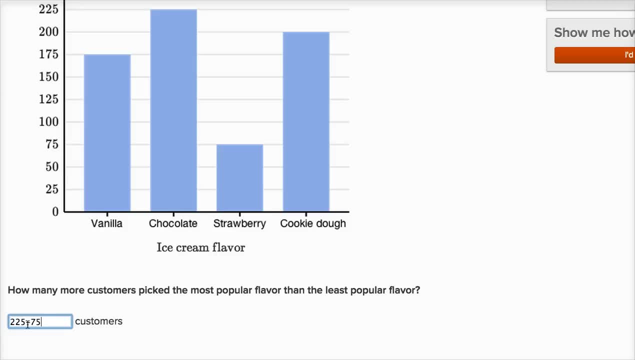 Minus 50 would be 175.. Minus 75 would be 150.. So we get 150 customers And once again we're saying that 150 more customers picked chocolate- the most popular flavor- than the least popular. Another way you could do it is you: 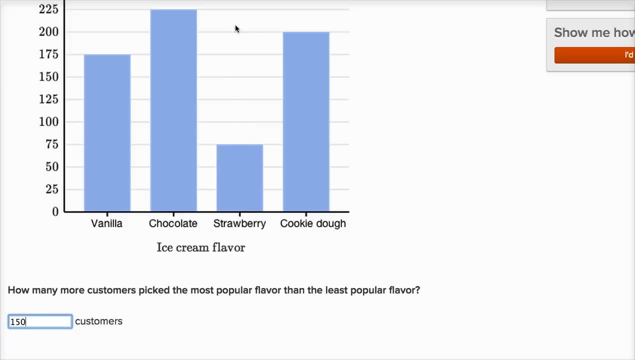 could look at the least popular and the most popular and say: well, how many more do I have to add to the least popular to get to the most popular? And you see 25, 50, 75,, 100,, 125, 150.